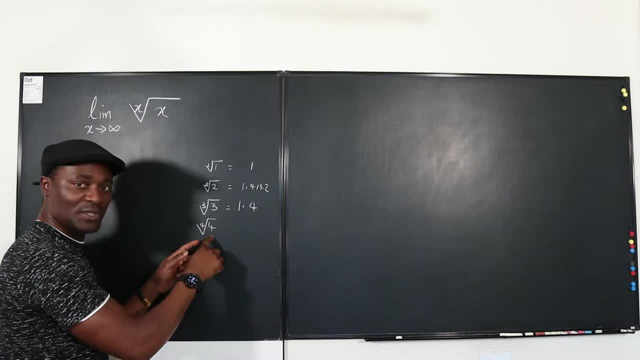 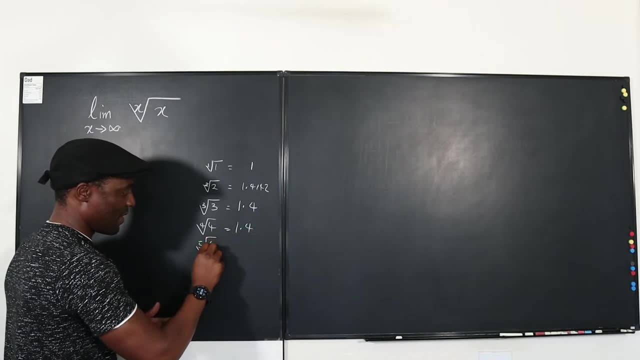 let's say 1.4. What about the fourth root of four? Well, the fourth root of four is the square root of two, So that's another 1.4.. What about the fifth root of five? It's going to be 1.3 something. 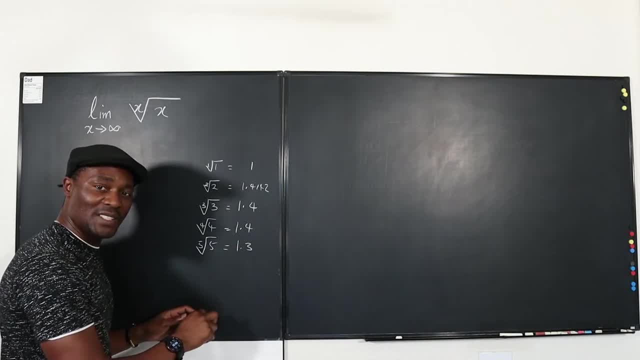 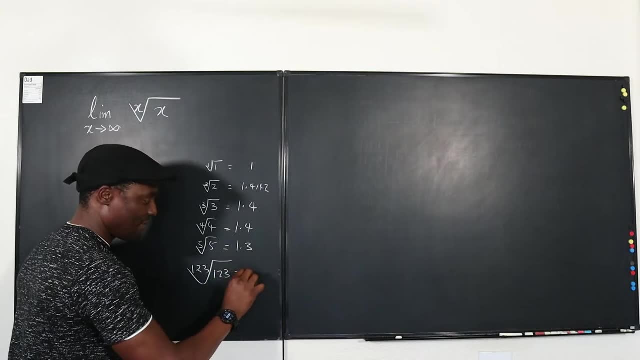 Okay, this is reduced. As you keep going you'll notice that the number gets smaller. So I tried 123rd root of 123, and I found my answer was 1.0, something. Okay, maybe 01 or 09,, I can't remember. 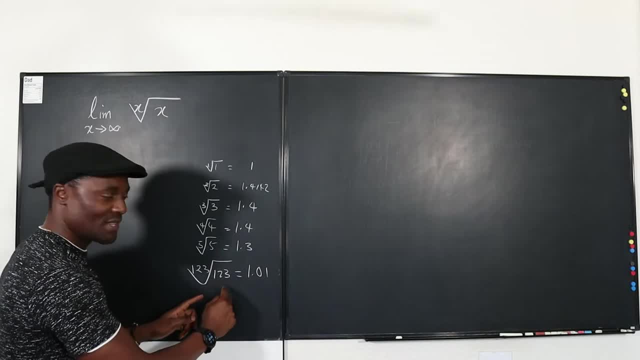 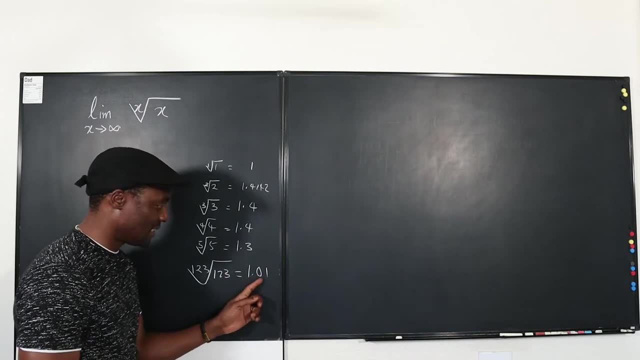 But you notice that as you keep changing these numbers, as it gets bigger, your answer approaches 1.. Now we don't know if it's going to go below 1, but it looks like this decimal keeps getting smaller, but the 1 is retained. 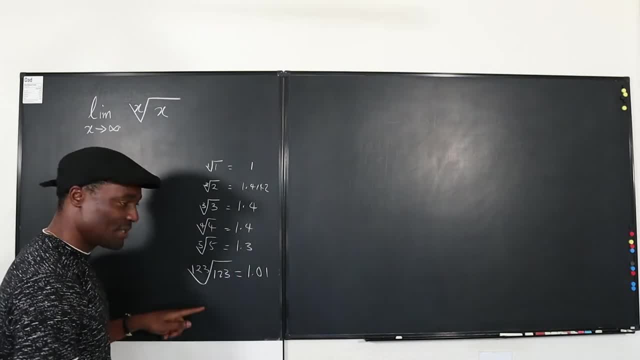 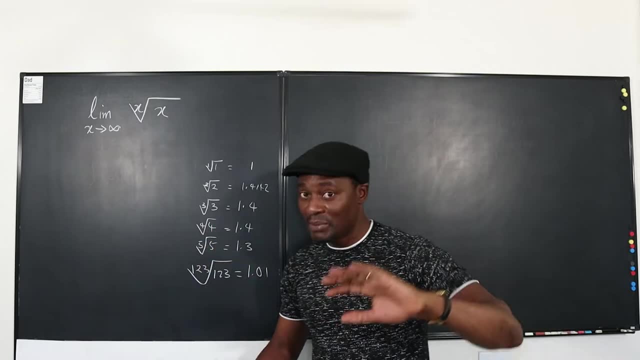 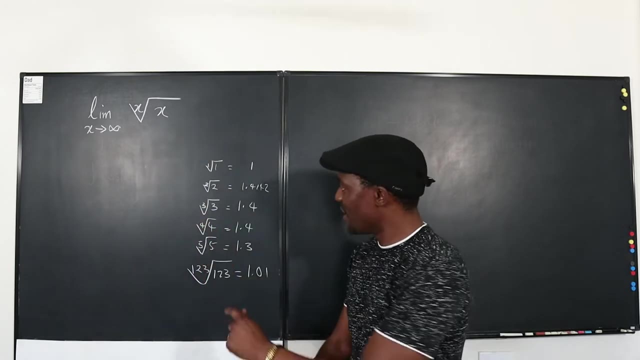 And that gives me an idea by observation, that as these numbers get bigger, you're going to get something like 1 at the end. So I can predict that by the time you approach infinity, your answer will be 1.. Okay, but you're not going to prove it this way, or you're not going to show it this way. 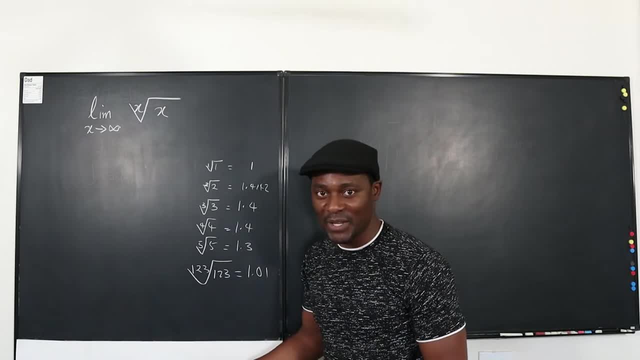 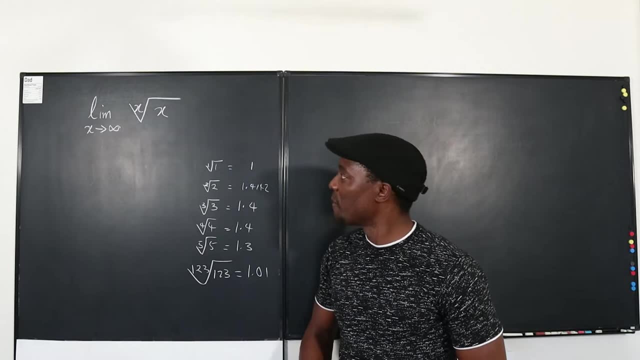 You have to show it mathematically and not by just making a table, Because you can't keep going until you get to just before infinity, which we don't know where. that is Okay, so let's do the math, the algebra of this. apply some rule. 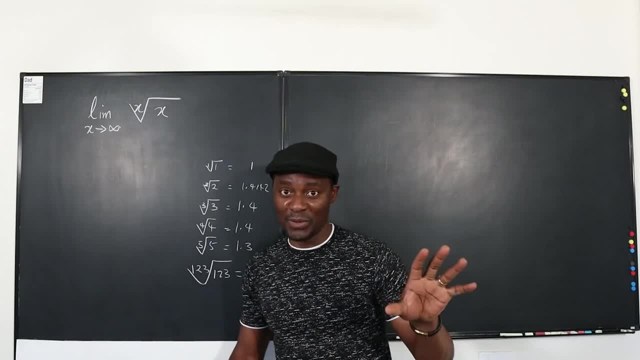 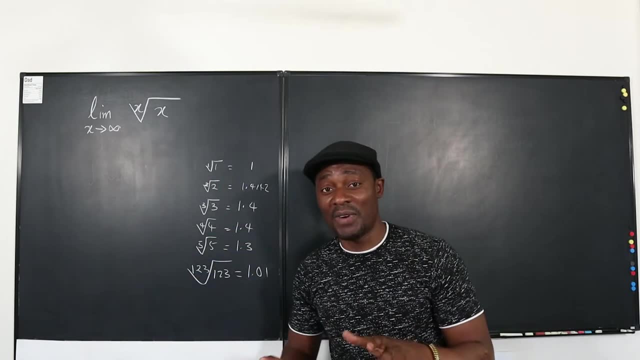 In fact, in this video I'm just going to show you where you can apply Lobito's rule and you can use that to solve this. But remember, this is an indeterminate form because you have infinity and infinity interacting And maybe it's too it's weird. 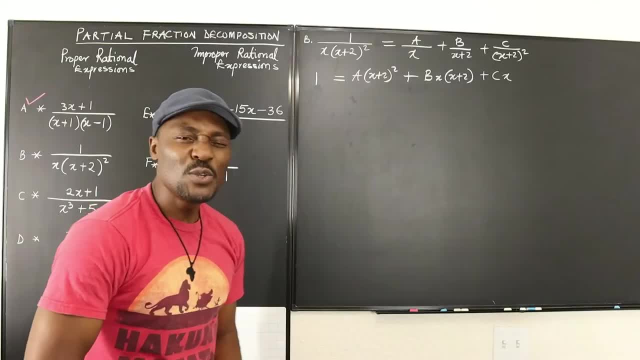 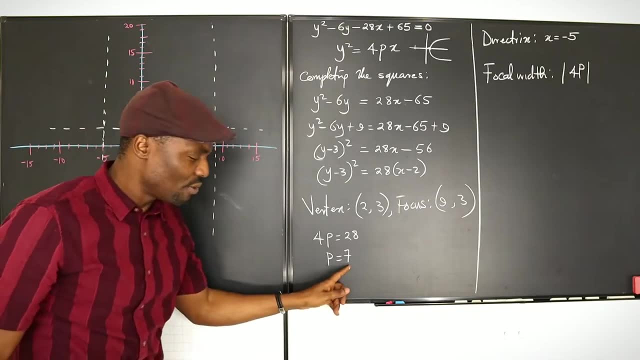 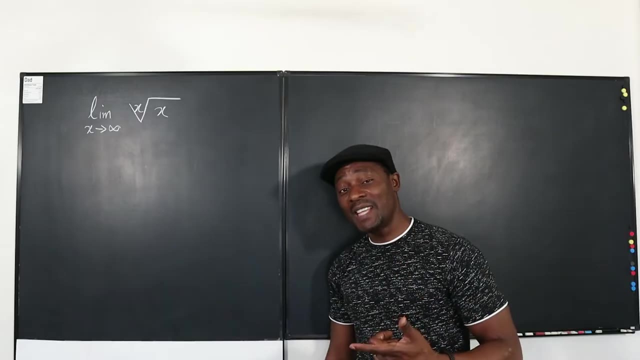 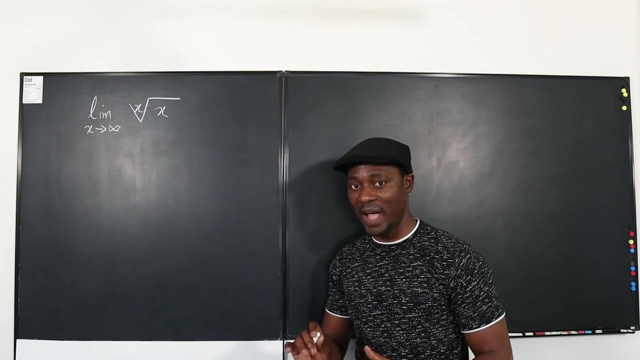 Okay, so let's rewrite this expression and see how it goes. Like I've said in other videos, whenever you see x approaching infinity, you must start thinking of how to make fractions out of whatever you have. Every time x goes to infinity, a fraction. 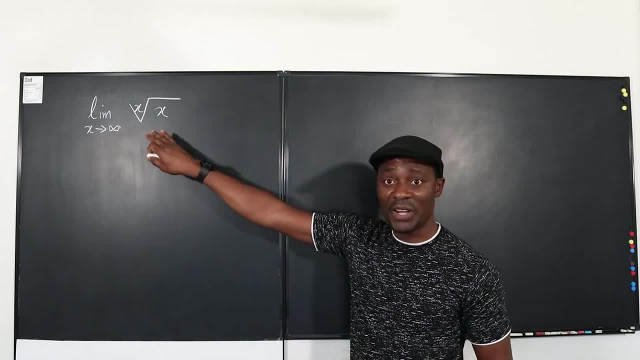 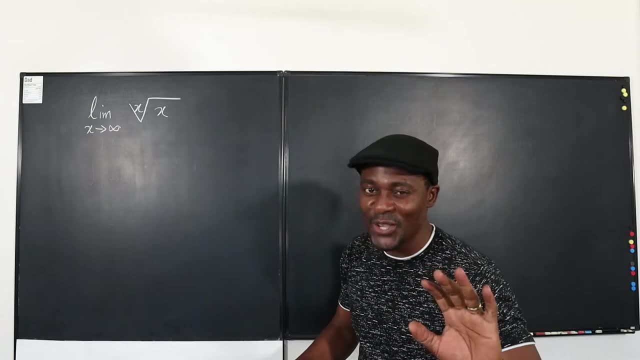 This will always save you, okay, unless it's so obvious, but right now it's not obvious. So whenever it's not obvious what's going to happen as you go toward infinity, it's always good to make fractions. So the first thing you want to do is rewrite this expression, not as a radical, but as an exponential function. 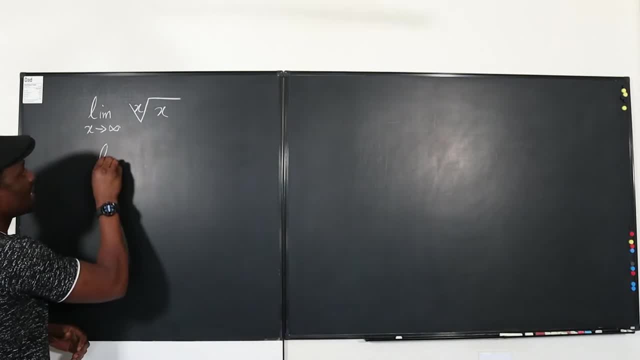 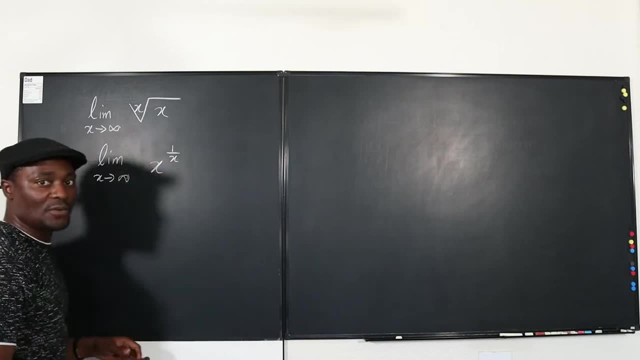 Okay, so let's look at this. We can say: this is the same thing as the limit, as x goes to infinity, of x to the 1 over x. That's another way to write this. Okay, remember that if you write x. 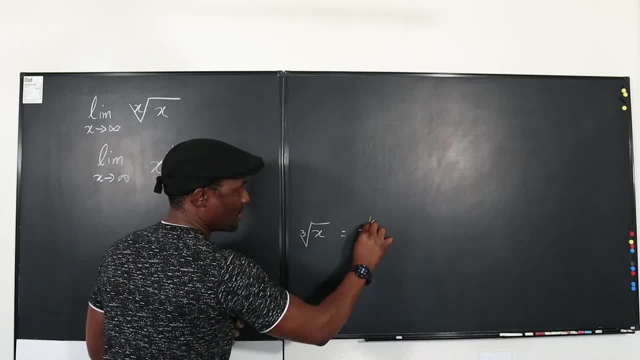 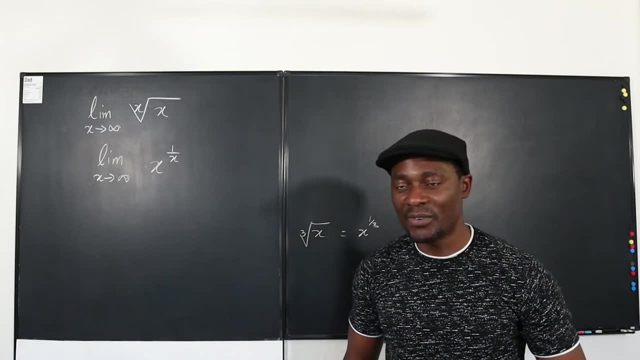 the cube root of x can be written as x to the 1- 3rd- the same thing. So that's what we just did here. Now we don't want an exponent, We want a fraction. Right now, we still have an exponential function. okay, a complicated one, for that matter. 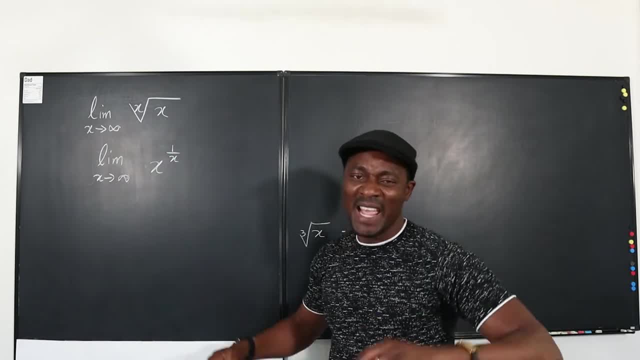 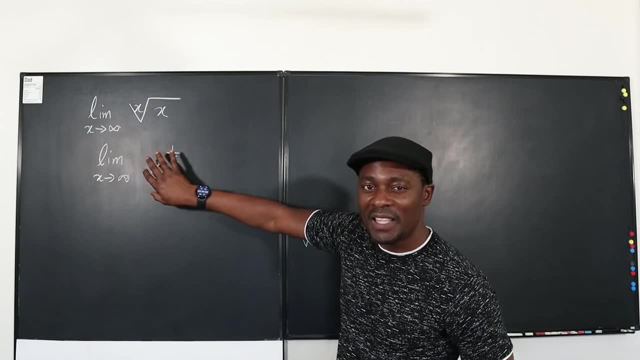 So what you want to do is rewrite this expression so that it is a fraction. You just want a fraction. Now, every time there's an exponential function, you want to take the natural log of it. okay, So if we take the natural log of it, 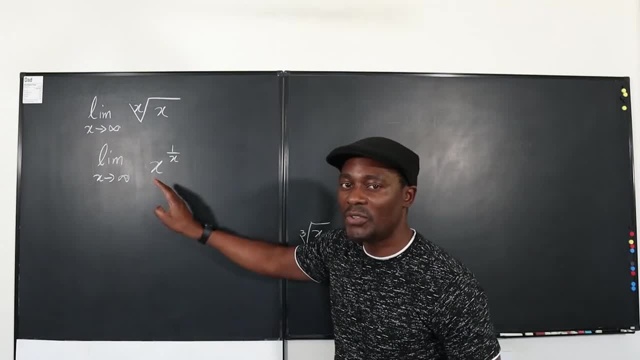 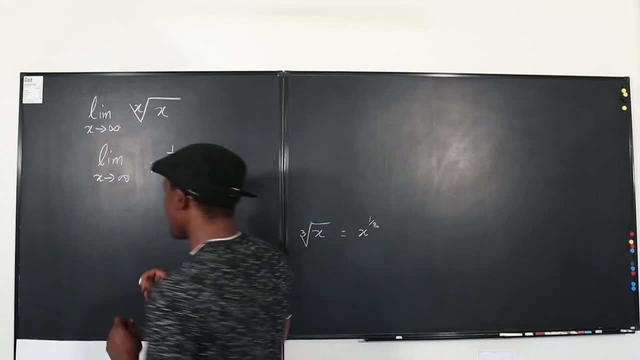 it makes your life a lot easier. But if you take the natural log, you have to undo the natural log you just did, Otherwise you're changing the value or you're changing the question. okay, So we can say: this is the same thing as the limit. 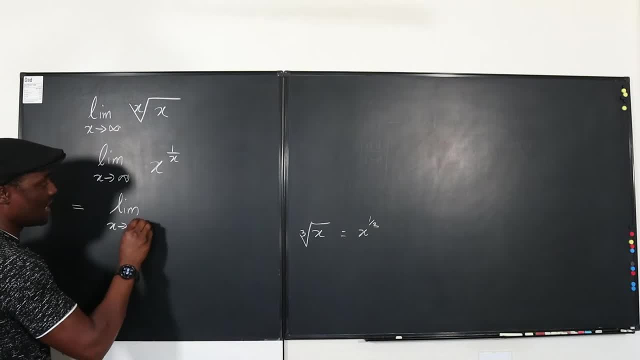 okay, the limit, as x approaches infinity, of if you take the natural log of this expression, you still have to take the e of it. Now watch what I'm going to do. I'm going to do two things: I'm going to express this in terms of e and then take the natural log of it. 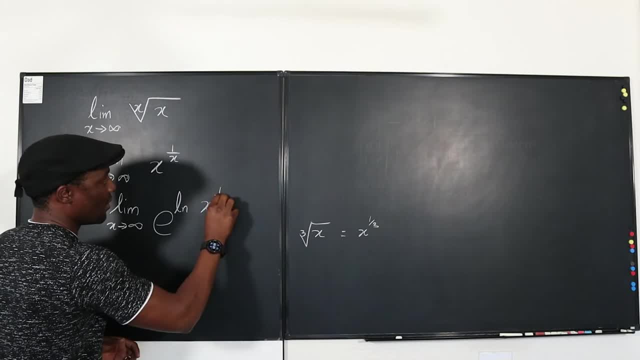 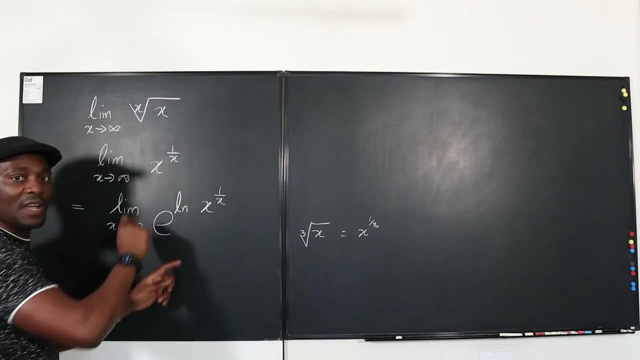 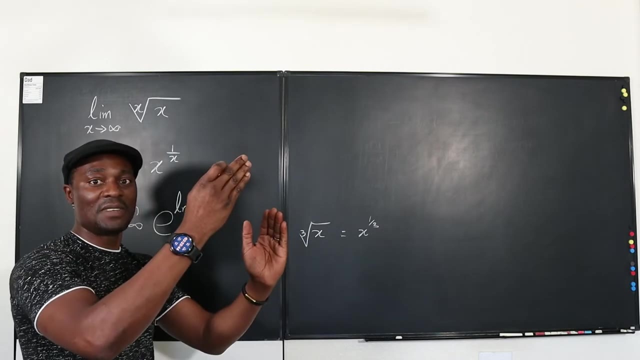 Okay, of x to the 1x. See, these two will cancel each other out and you still have what you have originally. but this just makes your life a lot easier. This is a trick you have to employ. Take the natural log, take the e of it immediately, and then you have. you still have this back. 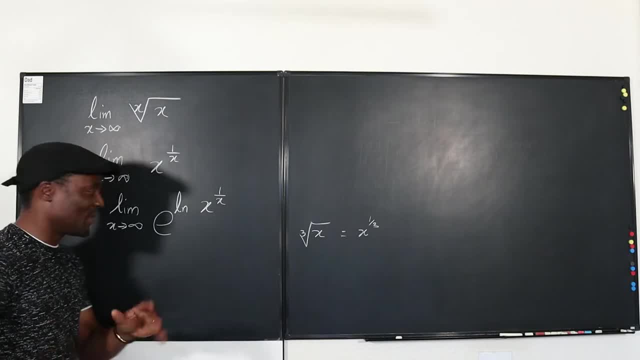 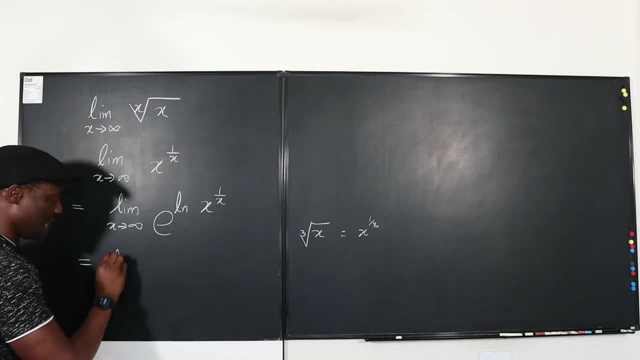 This is one of the laws of logarithms and exponential interactions. okay, Yeah, so here we go. Now we've got this. If you do this, what you have eventually is the limit, as x goes to infinity. of you see this, 1 over x can come down here. 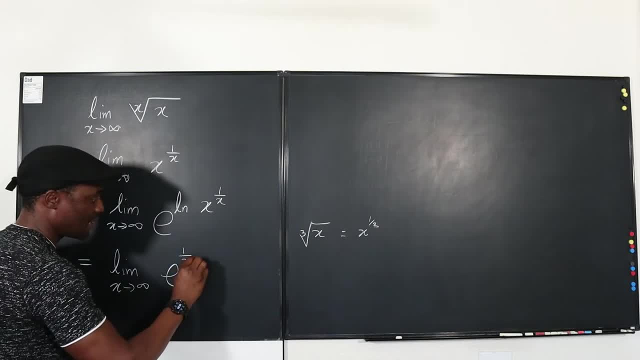 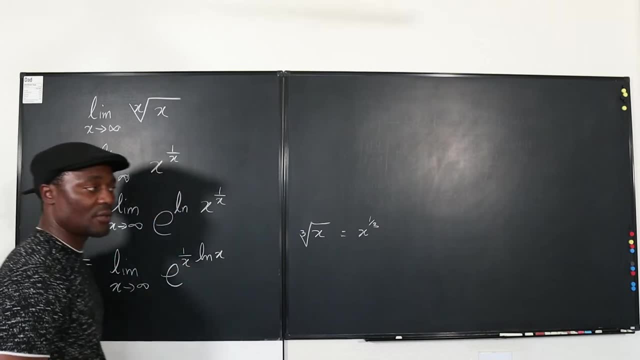 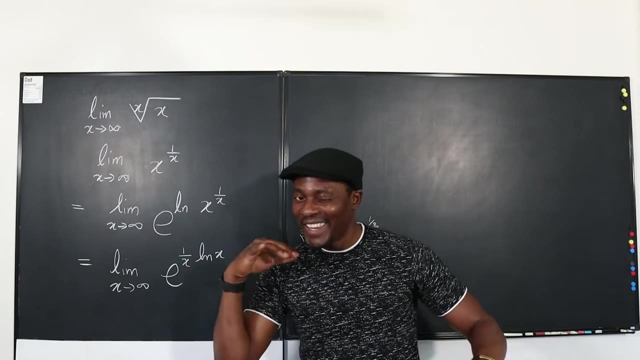 It's going to be e to the 1 over x natural log of x, because this can still go back and it can get back expression. So I haven't really changed anything, I just rewrote it in a way that makes sense. Now, this is where you need to remember some of the principles, right? 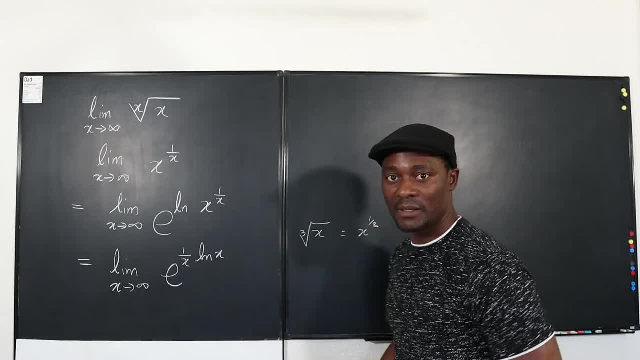 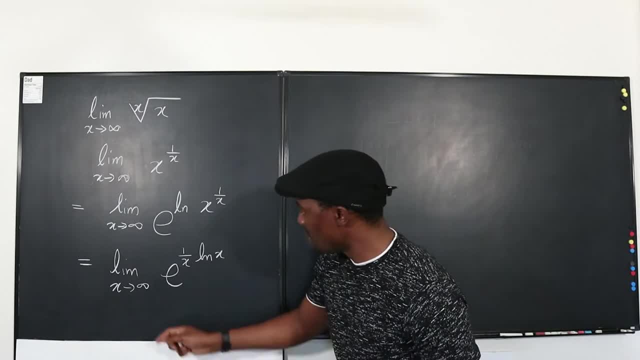 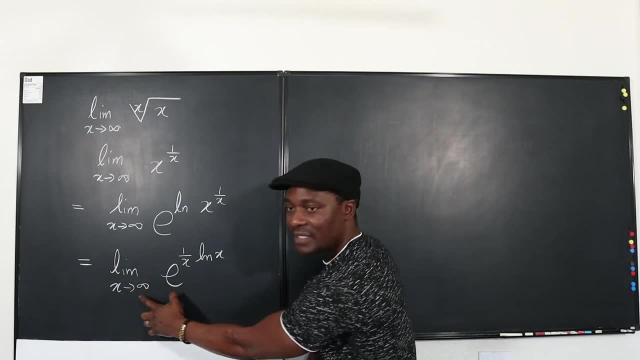 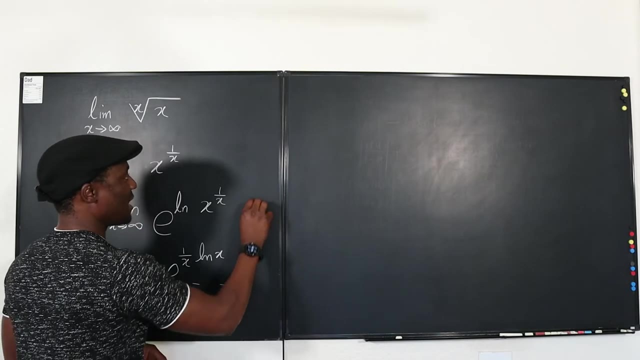 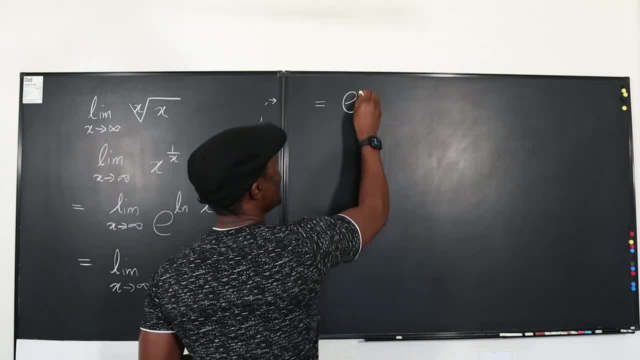 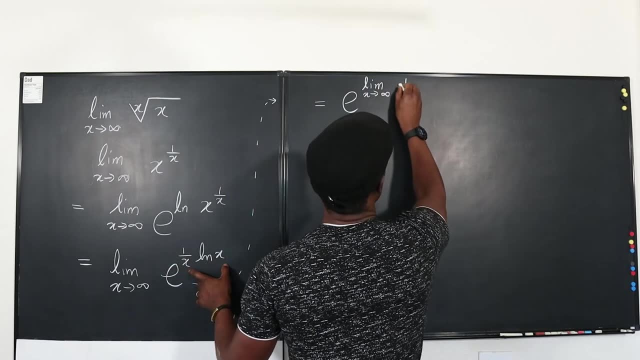 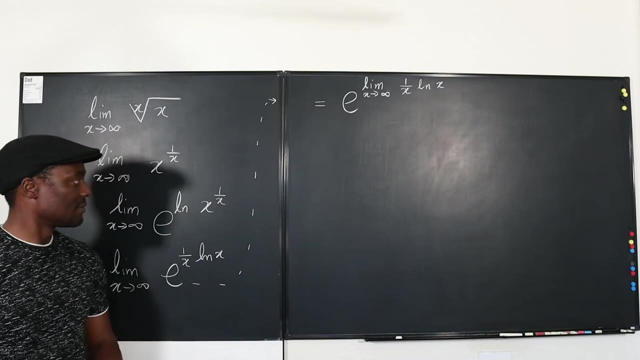 This expression. I can rewrite it as this: This is e raised to the limit. This is e raised to the limit As x goes to infinity of this expression. 1 over x of ln, 1 over x of ln. Do you see that? 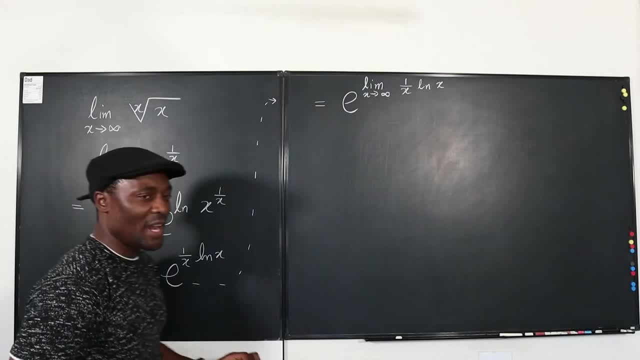 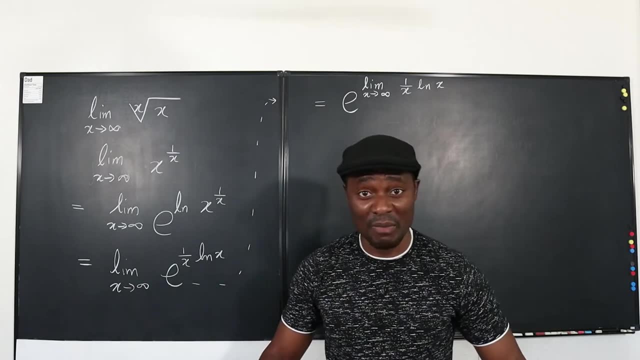 So I have moved this limit in here. Well, I tell myself that the limit of a function is the function of the limit. Okay, I just said that, so I can always remember: The limit of a function is the function of the limit. 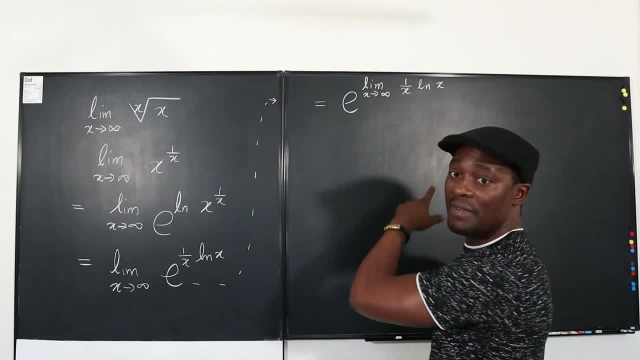 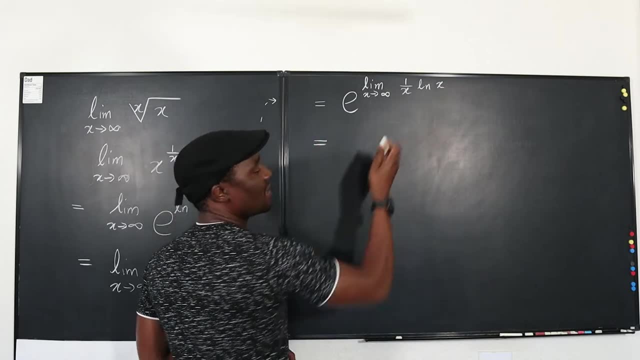 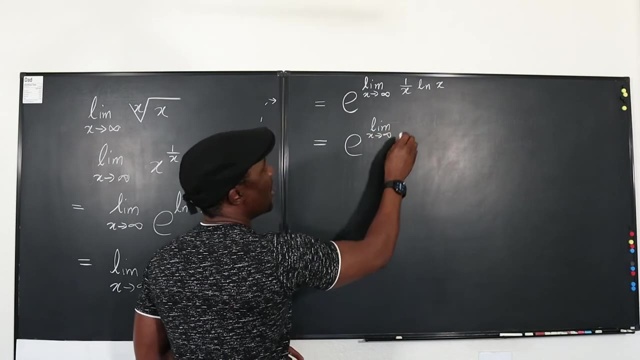 As long as in the limit that you have, That is not affecting anything, okay. So what you're going to do now is just simplify this. Take this limit- I'm sure you've seen this before. This is e to the limit, as x goes to infinity of. this is the natural log of x divided by x. 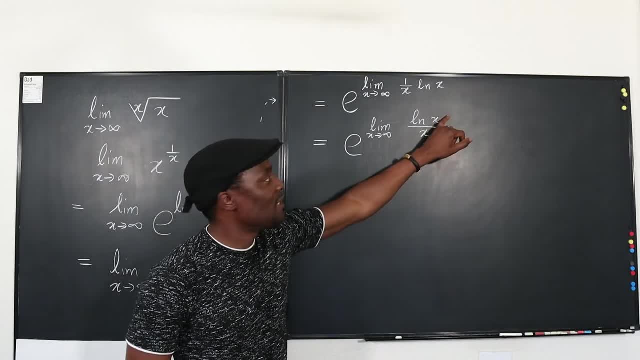 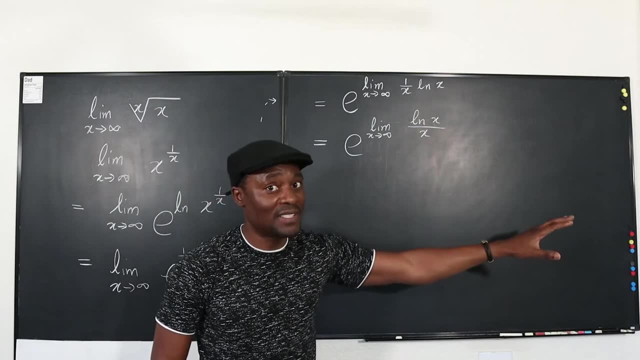 Okay now this actually is more or less an infinity over infinity case, Because as x goes to infinity, ln of x goes to infinity, That's certain, okay. And as x goes to infinity, x goes to infinity. So this is an infinity over infinity case. 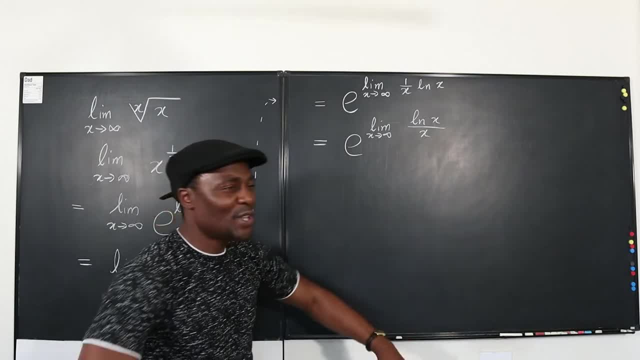 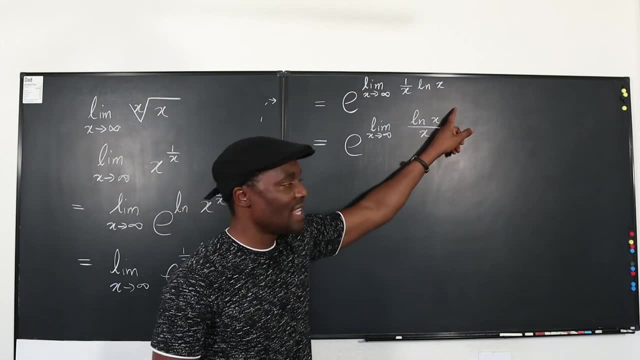 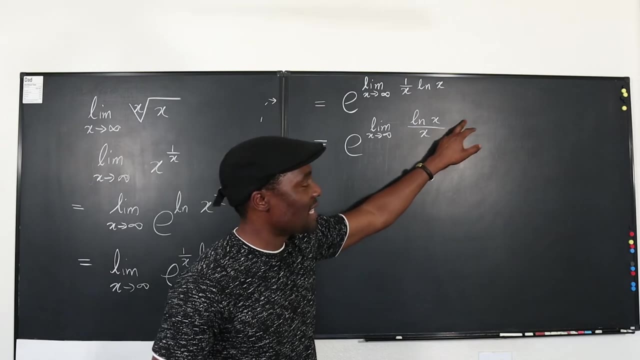 So Lobito's rule will work here, okay. However, you can also observe that, as the natural log of x, as x gets bigger, yes, this is increasing, but it's increasing at a slower rate compared to x. Therefore, as this gets bigger, this also gets bigger. 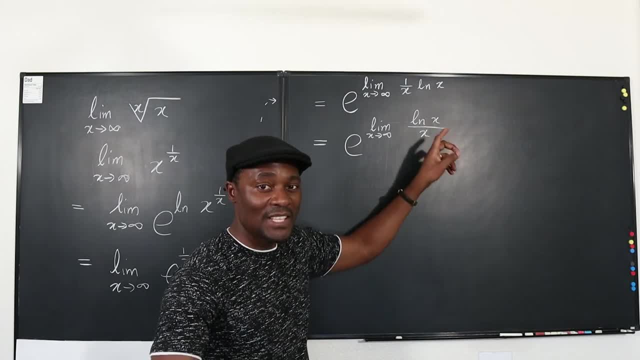 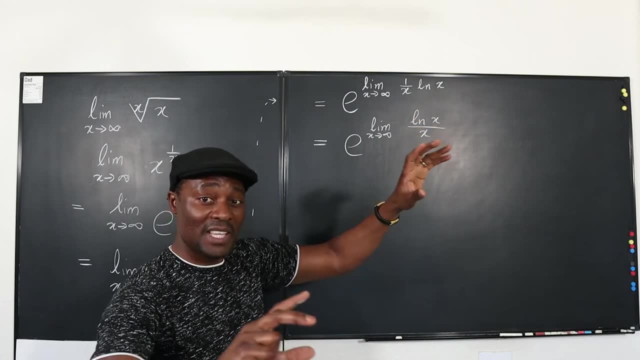 But because this is getting- It's getting bigger faster than this- it's going to go to zero. okay, If the numerator appears to be smaller compared to the denominator, as the denominator gets larger and larger, the expression goes to zero. So this expression goes to zero. 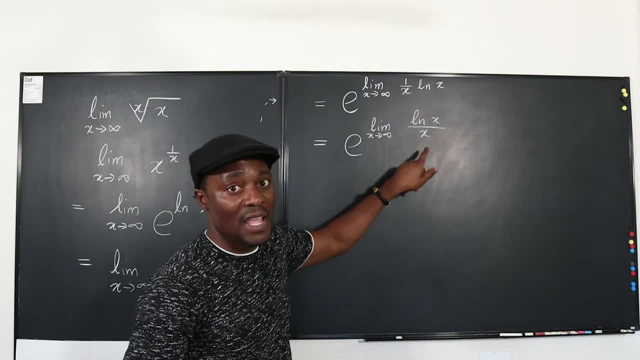 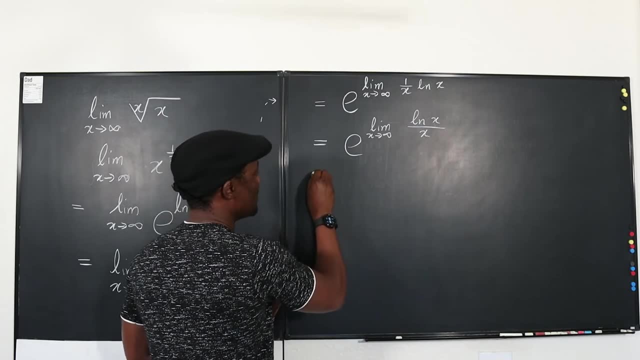 However, you could apply Lobito's rule. Take the derivative of the top and the derivative of the bottom and we're going to have: okay, let's apply So Lobito's rule, let's do Lobito's rule here.